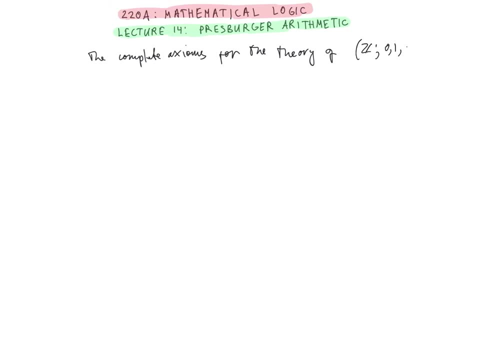 with the constant symbol 0,, 1, addition, subtraction and the linear ordering, But, very importantly, no multiplication. If we also had multiplication in the structure, then this would be a structure in the context of the Gödel's incompleteness theorem and we would know that there is no reasonable. 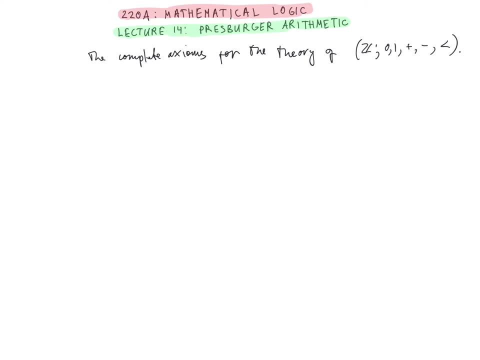 recursive axiomatization for the complete theory of the integers with addition and multiplication. However, it turns out that for addition alone there is a very nice description of the axioms of the theory And we have a very nice Quantifier-elimination result. 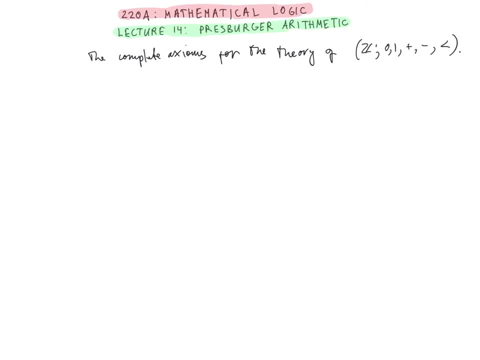 This also gives us a first example of a situation where, in order to obtain Quantifier elimination, we have to expand the language of the structure. namely, one can show that any quantifier-free formula, fís in the language L, consisting of the constant symbol zero, one plus minus less. 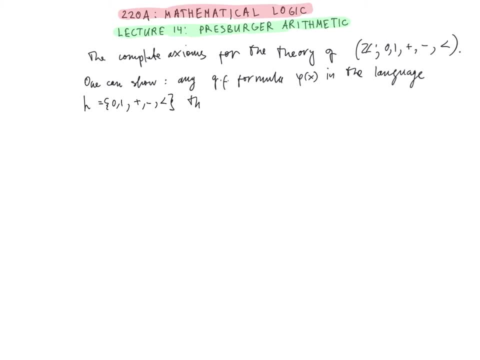 than So. for every such quantifier-free formula, in a single free variable X there exists a natural number n, such that either we have that the structure z together with zero, one plus minus less than satisfies phi of n, for all natural numbers n greater than capital N. 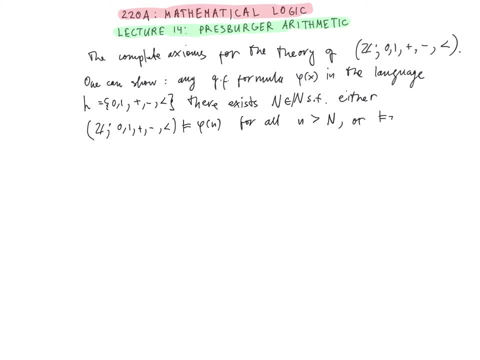 Or it satisfies the negation of phi of n for all n greater than capital N. So we see that every quantifier-free formula, the set of its solutions in the structure, is either final or co-final. In particular formulas such as, for example: exists y- x is equal to y plus y and exists y- x is equal to y plus y plus y, etc. 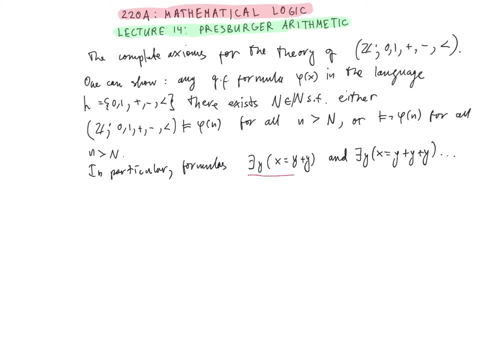 So the first formula defines the set of even integers. The second one defines the set of integers divisible by 3, etc. So these formulas are not equivalent to any quantifier-free formulas in the language L. So this can be verified as an exercise. 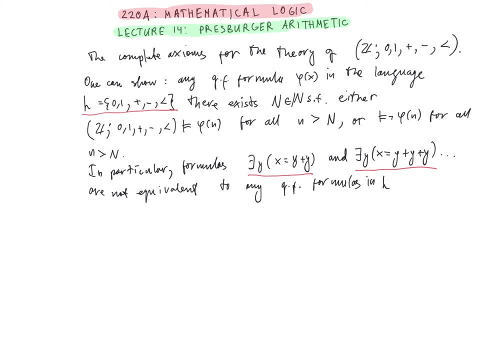 That every set defines. The set of integers definable in this language is either final or co-final in this structure, And so this suggests that in order to obtain quantifier elimination, we would have at least to expand the language by some new predicate symbols for this kind of formulas. 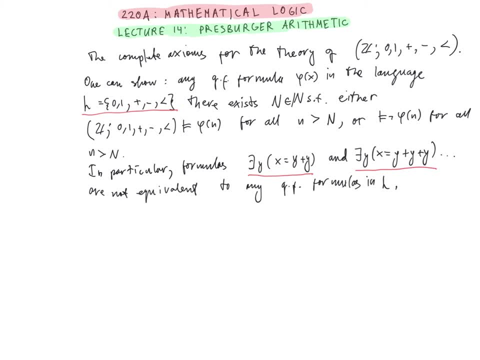 The important result of Pressburger is that, in fact, this is all that we have to add to the language. Towards this purpose, we consider the language LPRESB, Pressburger To be all the symbols from L, And we also add new unary predicate symbols p1,, p2, etc. 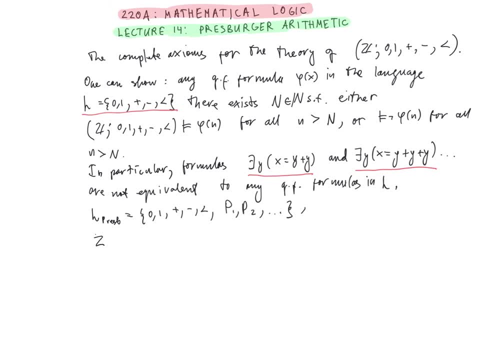 Next we expand the structure on the integers to the structure z tilde With the underlying base set the integers, The constant symbol 0,, 1.. And addition, subtraction less than all, interpreted as usual, And the predicate symbols pi are interpreted as z, 2z, 3z, etc. 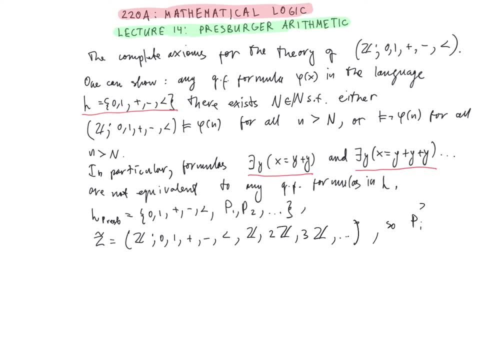 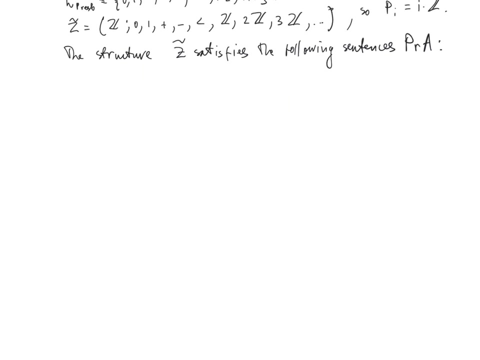 So pi is interpreted in z tilde as the set i times z, So all the integers divisible by i. Then the structure z tilde satisfies the following set of sentences, which we denote as PRA for Pressburger arithmetic. So we have 1.. 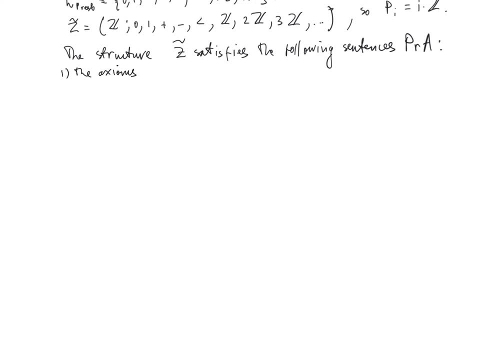 The axioms of abelian groups For addition and subtraction. Now the axioms expressing that The ordering relation is a linear order. 3. For all x, y, z. x is less than y implies that x plus z is less than y plus z. 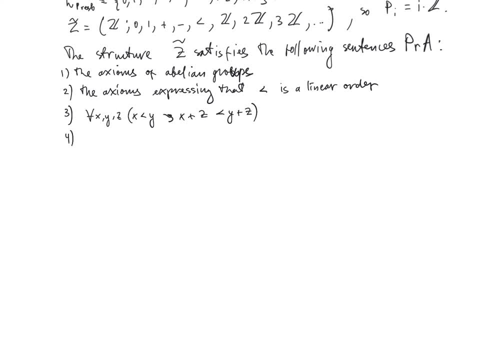 So the operation of addition respects the ordering 4.. We have 0 is less than 1. And there does not exist y, Such that 0 is less than y is less than 1.. So the discreteness axiom for the linear ordering. 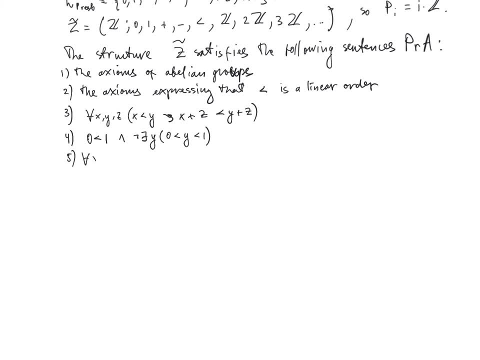 Next 5.. For all x exists, y- Such that Disjunction over all r Gratitude- Greater or equal than 0.. And less than n We have, x is equal to ny plus r times 1.. For n, a natural number greater or equal than 1.. 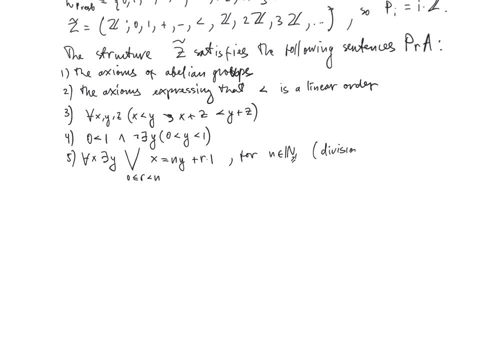 So this is the axioms expressing division with remainder. So for each fixed natural number n, Every element x can be divided by n with remainder. And finally, axiom 6. For all x, Pn, x, If, and only if, Exists y. 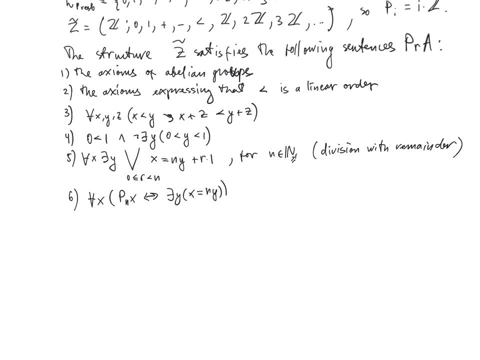 Such that x is equal to ny, Again, For every n Natural number greater or equal than 1.. So these are the axioms which define The interpretations of the predicate symbols: Pn That we add into the language That they express exactly. divisibility by n. 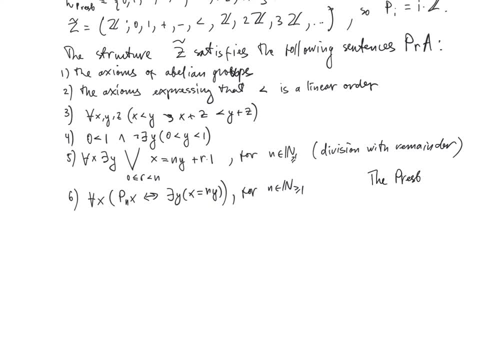 So these are the Pressburger arithmetic axioms And we are going to prove the theorem. Pressburger arithmetic has quantifier elimination Proof. Let Phi of x, 1 through xn, y Be a conjunction Of Atomic And. 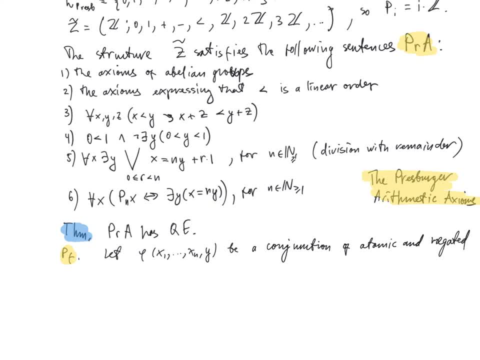 Negated atomic Formulas In the language LPRESB By our early discussion of quantifier elimination. We know that it suffices to show That The formula Exists. Y Phi of x Bar Y Is: 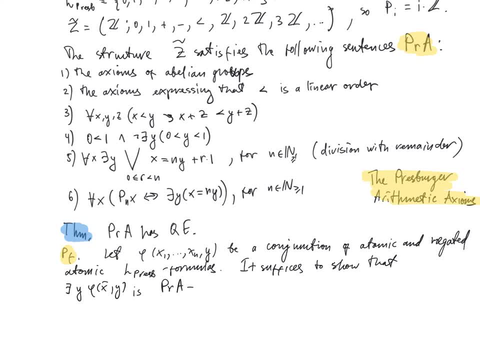 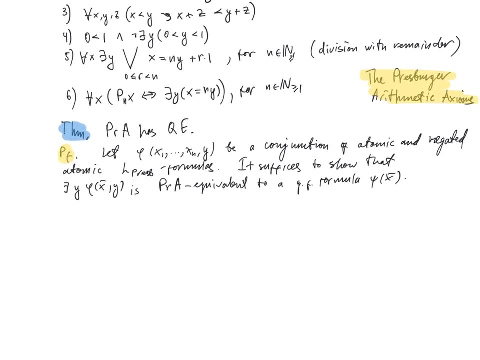 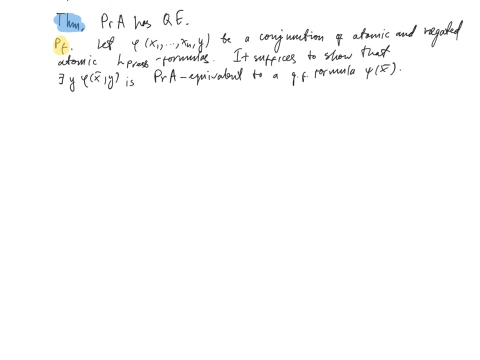 Equivalent In PRA To a quantifier free Formula, Psi of x, Bar. We begin by Trying to understand more explicitly What Such a basic conjunction, Phi, Looks like, Claim one. We may assume That 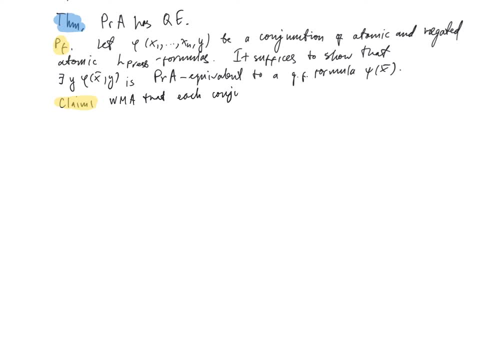 Each Conjunct Of phi Is One of the following, So of the following form: For some M N Natural numbers Greater or equal than one, And T Of x And L Pressburger term. 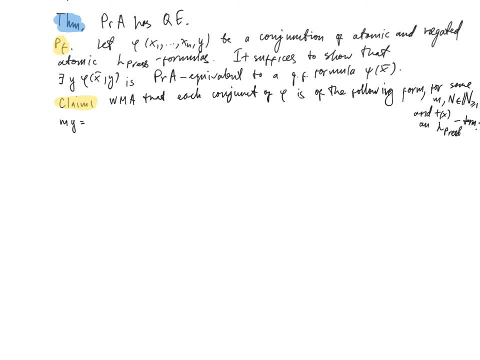 So the possibilities are: M Y Is equal to T Of x, M Y Is Less than T Of x, T Of x Is Less than M Y Or P N. 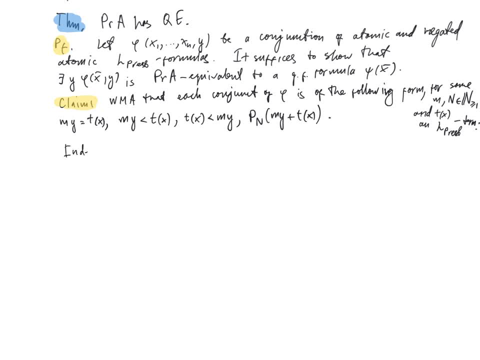 M Y Plus T Of x. Indeed, Every Conjunct Of the form M Y Is Not Equal To T Of x Can Be Replaced By The Formula: 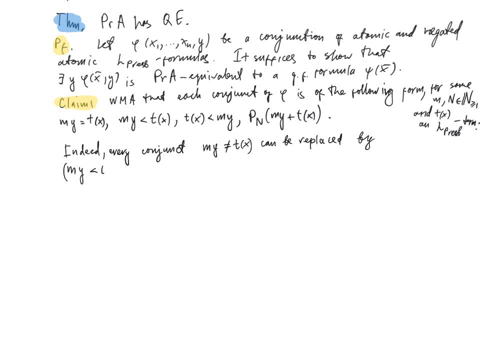 M Y Is Less Than T Of x, Or T Of x Is Less Than M Of y, Which Y Is Not Equal To T Of x, And. 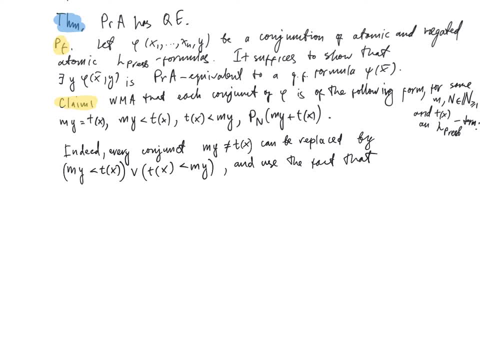 Then We Can Use The Fact That The Formula Exists: Y, Phi One Of X Y Or Phi Two Of X Y. So The Existential, 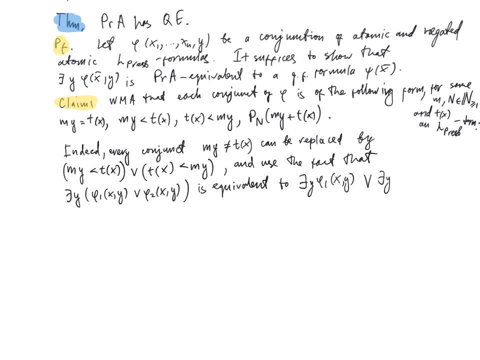 Quantifier Commutes With Disjunctions, And Hence The Formula Phi That We Started With In Disjunctive Normal Form Can Be Modified So That 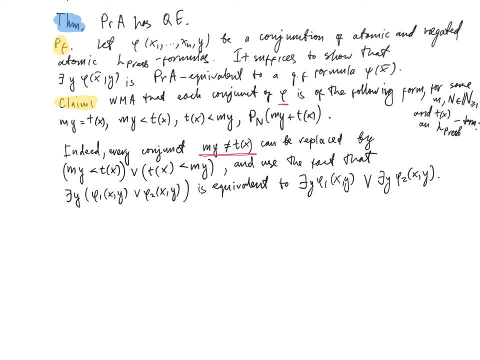 Every Term Of The Form Becomes Instead A Disjunction Of Two Terms Of This Form, But Now Only One Of Them Occurs In Any 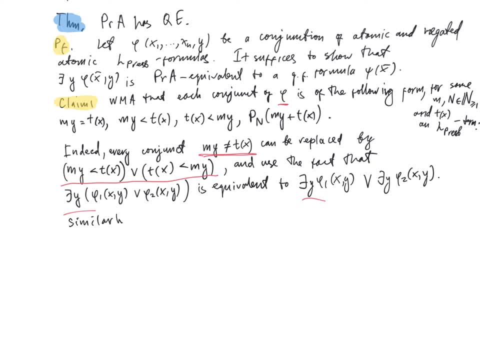 Given Conjunct Of This Formula And So Without. Also This Atomic Formula P? N Of M, Y Plus T Of X Can Be Replaced By: 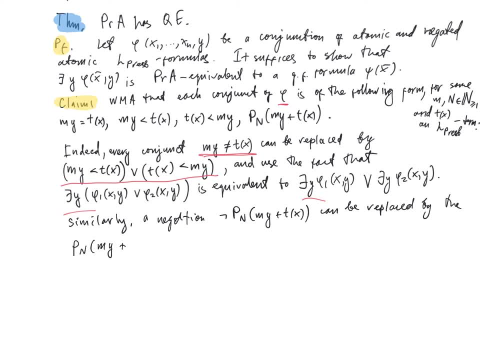 The Disjunction P N Of M Y Plus T Of X Plus One Or T Of X Plus N Minus One Times One. Let Us 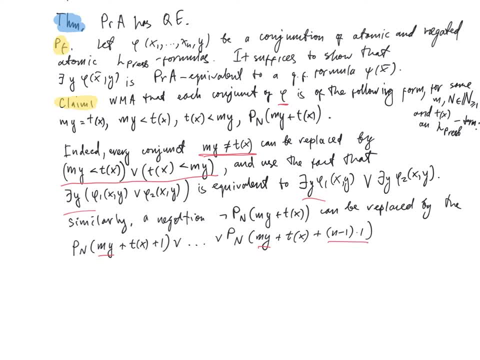 Be Clear Here And Throughout. We Don't Have Multiplication In The Language, So Every Term Of The Form, Of The Structure, And So We See. 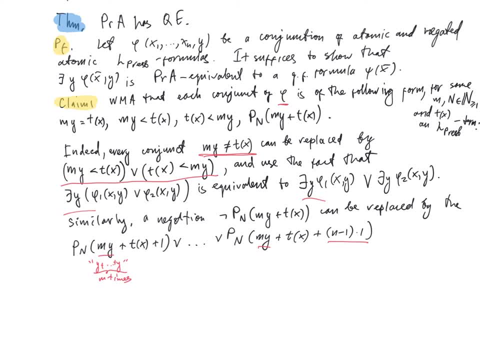 That Not Being Divisible By N Is Equivalent To Having One Of The Remainders Between One And N Minus One, Which Is All The. 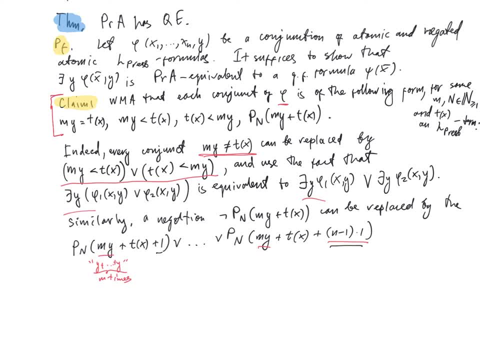 Possibilities For The Atomic And Negated Atomic Formulas, Where We Manage To Replace Every Negated Atomic Formula By One Of The Atomic Formulas. 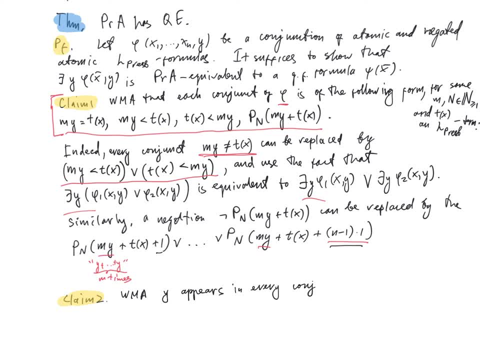 On This List. So Indeed, Conjuncts In Which White Doesn't Appear Can Be Eliminated Because We Have The Valid Sentence. Exists Y Psi. 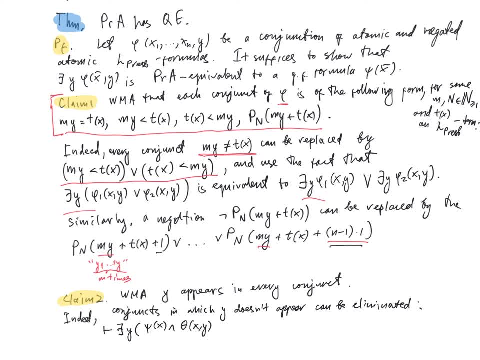 Of X And Theta Of X- Y Is Equivalent To The Formula Psi Of X. Conjunction Exists Y, Theta Of X, Y. So We Have: 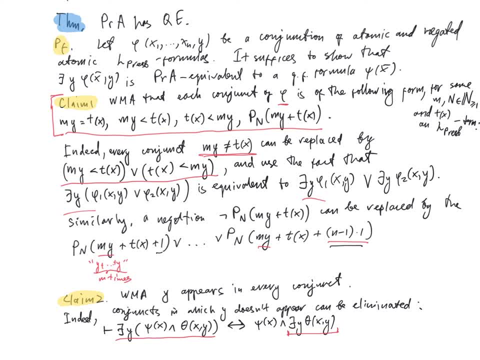 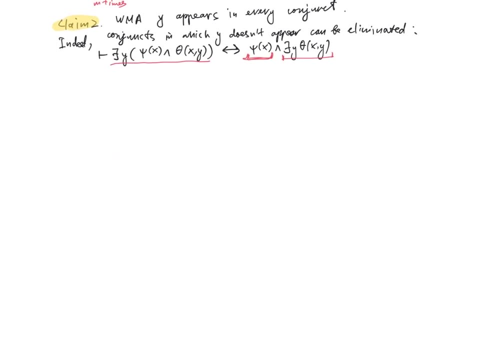 To Find In Quantifier Free Formula Equivalent To The Formula Exists Y, Theta Of X, Y For Any Psi And Theta. Since This Is Already. 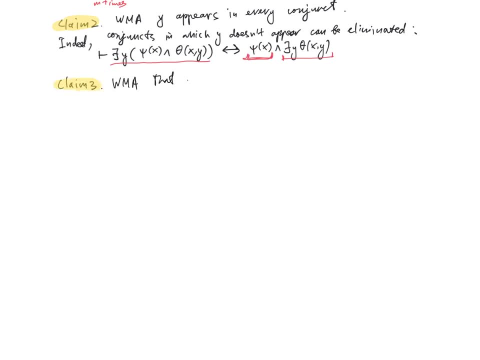 Quantifier Free This: All Conjuncts Have The Same Coefficient M In Front Of The Variable Y. Indeed, Since All Conjuncts Have The Same, 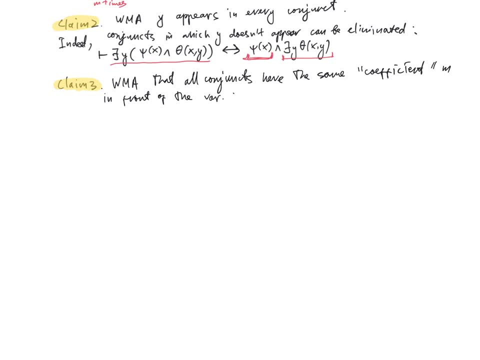 Coefficient M In Front Of The Variable Y. Indeed, Since Pressburger Arithmetic Implies That P N Of Z Is Equivalent To P R N, 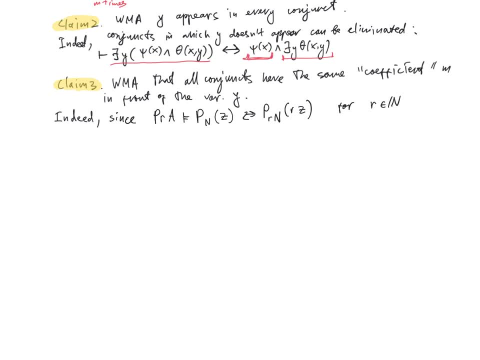 Of R Z For Any R A Natural Number Greater Equal Than One. We Can Replace P? N Of M Y Plus T Of X By. 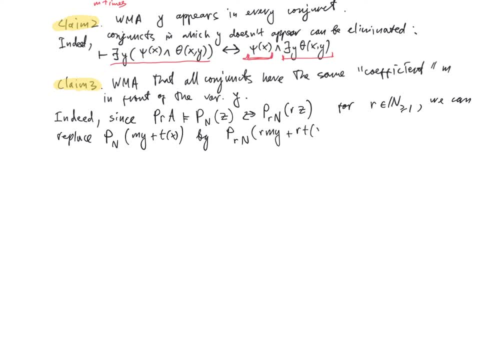 The Predicate P R N R M Y Plus R T Of X Also For R M Y, Is Equal To T X By R M. 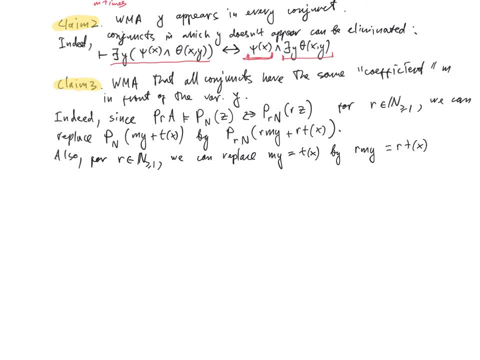 Y Is Equal To R T Of X, And Likewise We Can Deal With The Formulas Of The Form. T Of X Is Less Than. 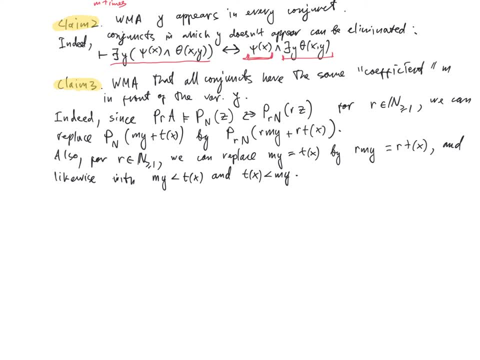 M Y, So Both Of Them. We Can Also Multiply Both Parts By R. The Logical Equivalence After Multiplying By R Is Guaranteed Of The 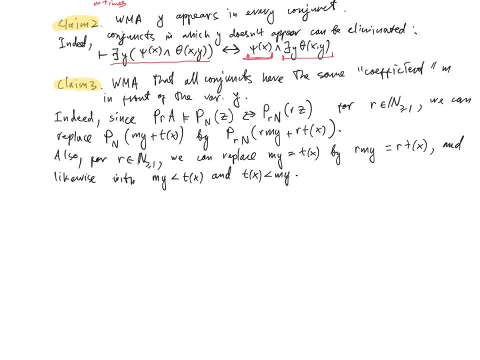 Coefficient That Appear, And, Using These Manipulations, We Can Change The Formula To One Which Is Equivalent In Pressburger Arithmetic And Has The Same. 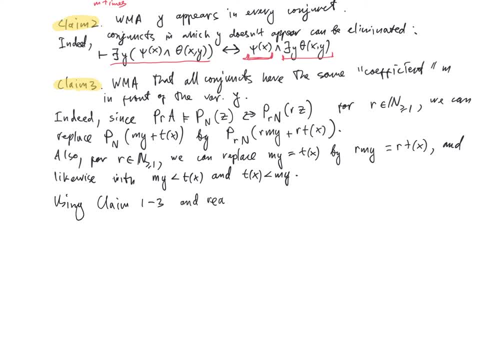 Coefficient In Front Of The Conjunction Over H In H And Y Is Equal To The Term T, H Of X And Conjunction Over 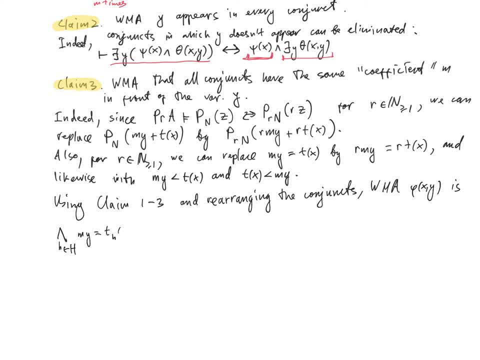 All I In I And Conjunction Over All I In I Of X Is Less Than M, Y And Conjunction Over All J In J. 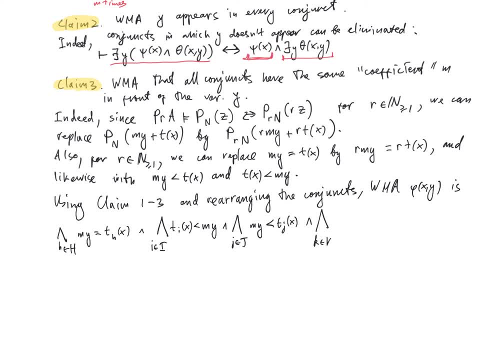 M Y Is Less Than T J Of X, And Conjunction Over All K In X Is Less Than M Of X And All Y. 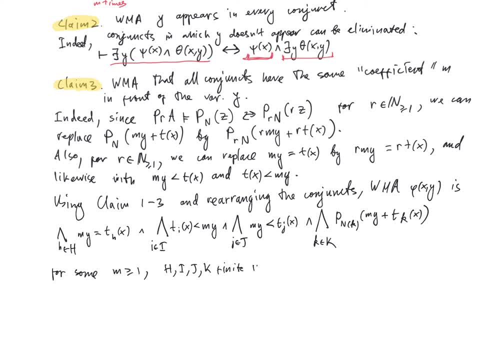 Is Less Than M Of X And M Is Less Than All. Y Is Less Than M Of X Is Less Than Of Y. M Is. 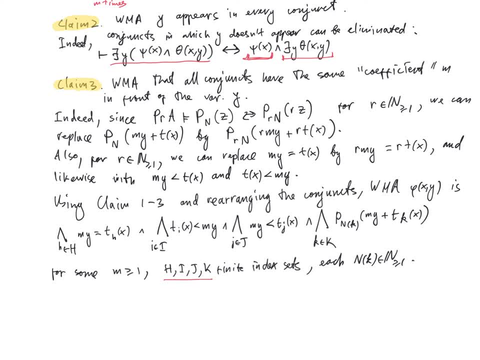 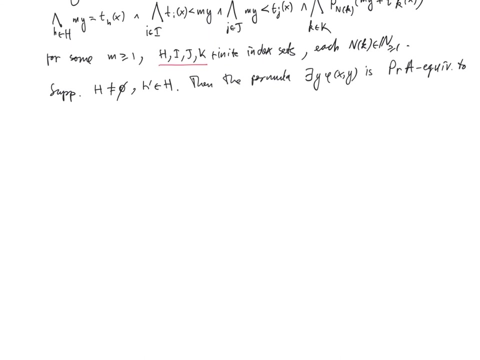 Less Than All. Y In. X Is Less Than M Of. X Is Less Than Of. Y Is Less Than X Is exists. y phi of is equivalent in Pressburger arithmetic to the following formula: 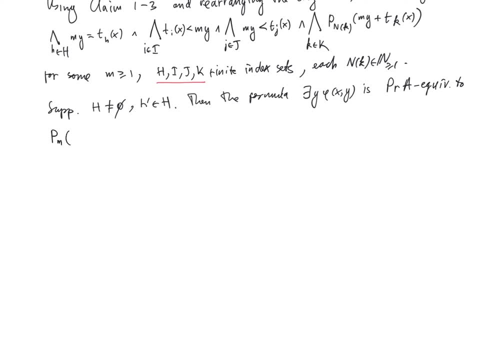 So we have p? m of t h prime of x and the conjunction overall h in h. t h of x is equal to t h prime of x and conjunction overall I in i. t i of x is less than t h prime of x. 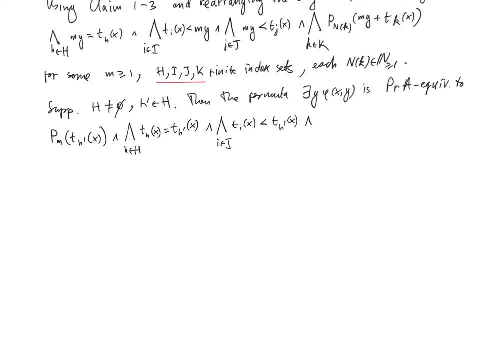 P? m of t? h prime of x. So we have p? m of t? h prime of x and the conjunction overall of X and the conjunction over all J and J. TH prime of X is less than TJ of X. and finally, 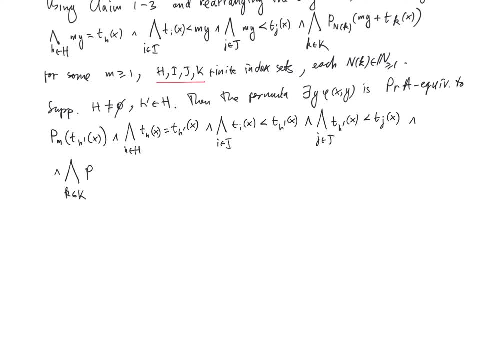 the conjunction over all K and K, PNK of TH prime of X plus TK of X. Let's see why this is true. Well, so, by assumption, if H prime is an H, we must have that the corresponding term TH prime of X is equal to MY. this is expressed by the first conjunct. 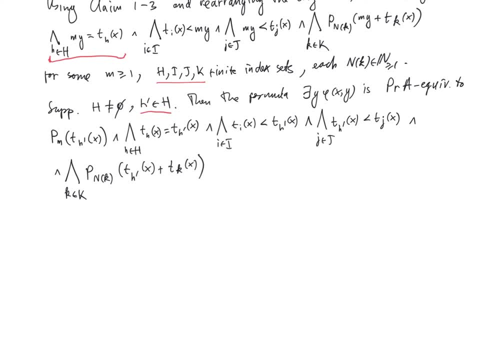 And the whole conjunction is satisfied, if, and only if, all of the conjunctions are satisfied. Hence, we might simply replace every appearance of MY in the formula by the corresponding term TH of X, which is exactly what we've done here, And in this way we obtain a formula without quantifiers which is equivalent to the original. 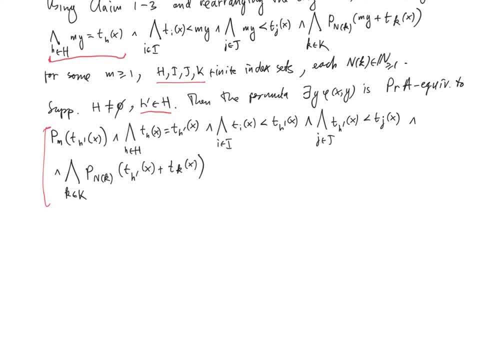 formula exists, Y phi of XY, So in this case we are done. Hence claim 4, we may assume that the set H is empty. So there are no conjuncts of this form expressing that MY is equal to a term of X. 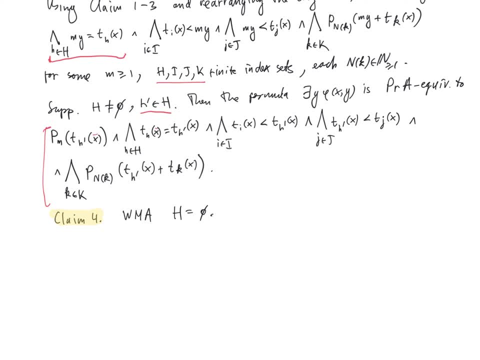 Let us also remark that we stopped writing the bar on X bar everywhere, so that's assumed. So X and X bar are not the same. The set H is the set of variables X1 through Xn. To understand the next step, we first focus on the standard model of Pressburger arithmetic. 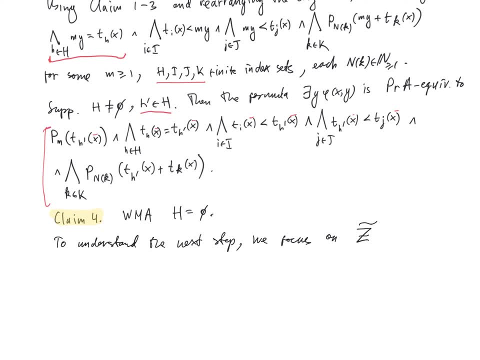 namely the structure Z, hat with the underlying set the actual integers, although the argument that we provide, In this case the set H, works in any model of Pressburger arithmetic. But first let's discuss it in the context of the usual integers. 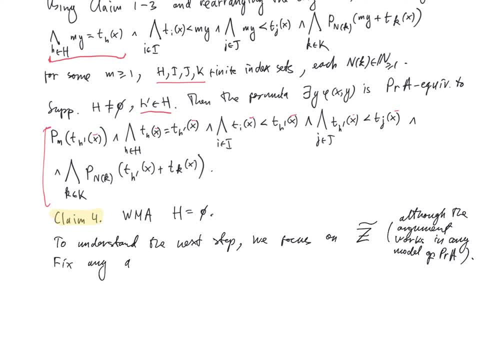 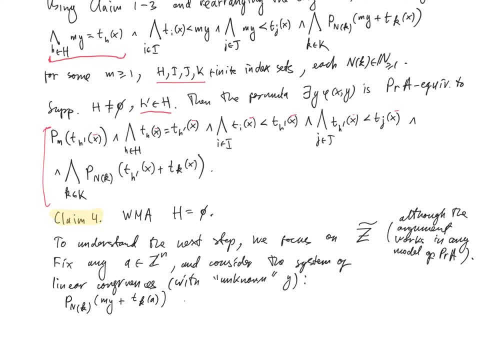 A for each K in K. So K is a finite capital, K is a finite set. So we have finitely many conditions like this on Y: Once the tuple A is fixed, which is more familiarly, can be rewritten as MY plus TK of A. 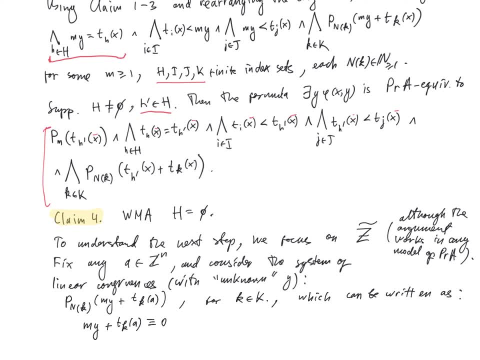 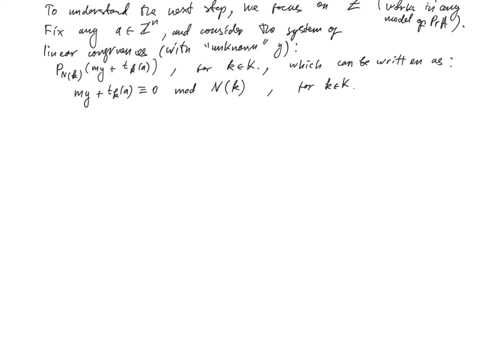 is congruent to 0 mod the natural number N of K, Which, again, we have one condition of this form for each little k in the finite set capital K. Now, given such a system of congruences, we know that the solution 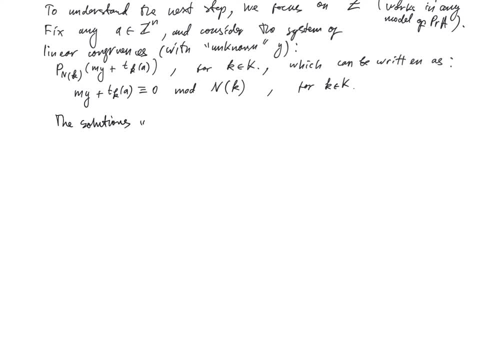 is a finite set In Z of this system form a union of congruence classes modulo the integer N, which we take to be the product of all of the NK For K in the finite set capital K, Since, of course, knowing the congruence class. 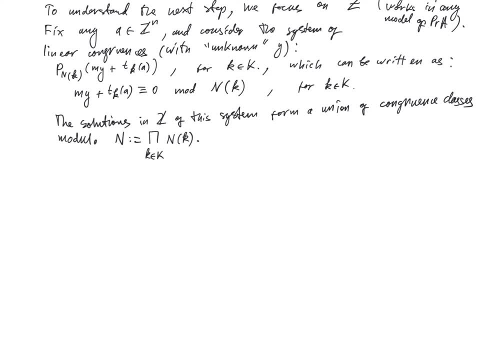 of an integer. with respect to this number, capital N determines the congruence class with respect to N of K for each K, Where, as usual, we put N, is equal to 1 for the case when K is there. So this is the empty set. 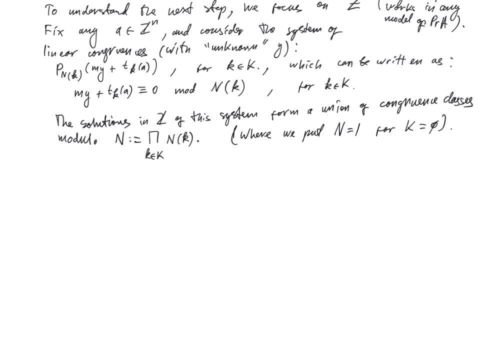 Now observing this situation over the integers. This suggests replacing Y successively by N Z, 1 plus N Z, etc. through N minus 1, and we have the final function And we can easily find out that the function N is equal to 1.. 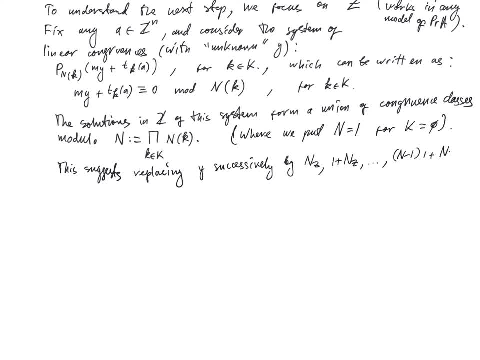 1 times 1 plus nz, instead of just quantifying over y. So our precise claim suggested by this discussion is claim 5.. The formula exists, y, phi of x. y is equivalent in Pressburger arithmetic to the formula theta of x, given by the following expression: So we have a large. 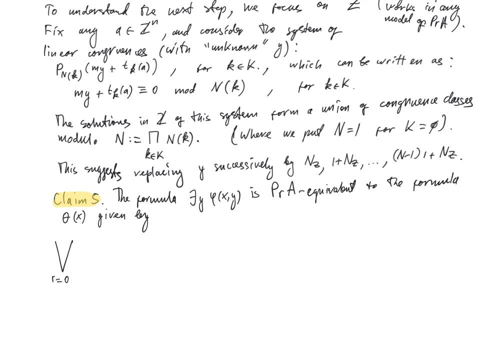 disjunction over all r from 0 to n minus 1, where again the capital N is the product of n of k that appear in the formula. Then we take the conjunction over all k in k, p, n of k, m, r times 1 plus tk of x, and there exists: 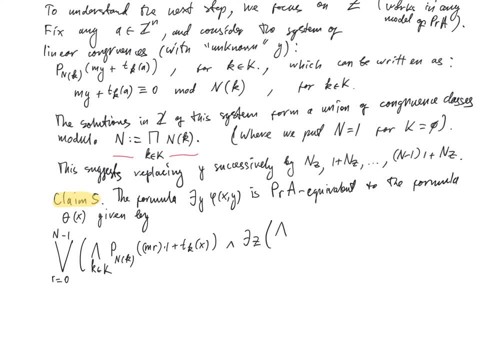 z such that we have the remaining conditions. So we have from the formula phi. So we have the conjunction over all k in k, p, n of k m r times 1 plus tk of x, and there exists z such that we have from the formula phi. So we have some. 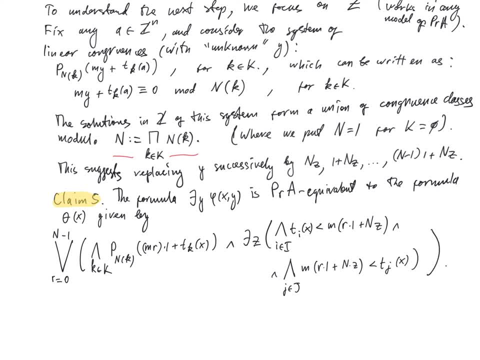 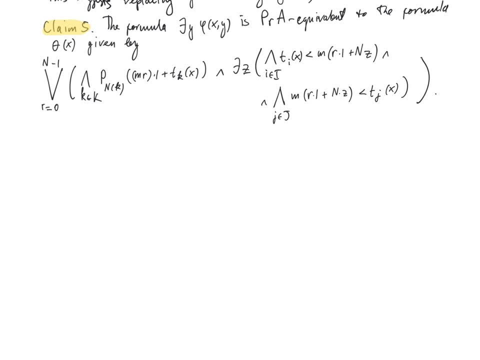 privileged predictions. It's meet with n times 45 and one plus. let's theoretically apply to supposing this case. Now, if the last x was m, then If the last x was passed, deteriorating into the next vy. we Note that the quantified variable is no longer subject to the congruence conditions as we 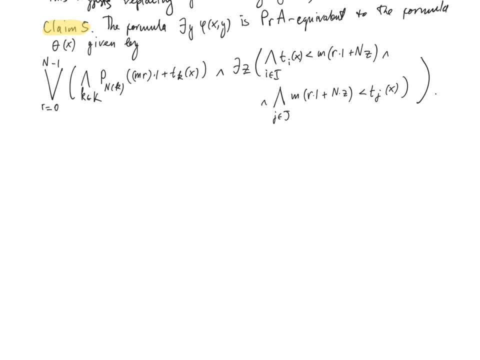 originally had in phi, since we can replace it by this new formula now. Proof of claim 5.. Proof that A with the base set A is an arbitrary model of Pressburger Arithmetic and we have the tuple A consisting of A1 through An from the base set capital A. 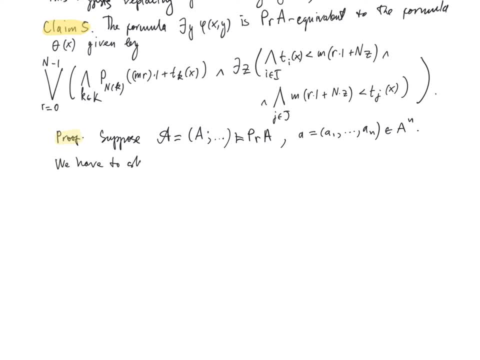 Now we have to show that a, b, c, d, that A satisfies, exists, Y, phi of A, Y if, and only if, A satisfies theta of A. So let B be an element of the base. set A such that A satisfies phi of A, B. 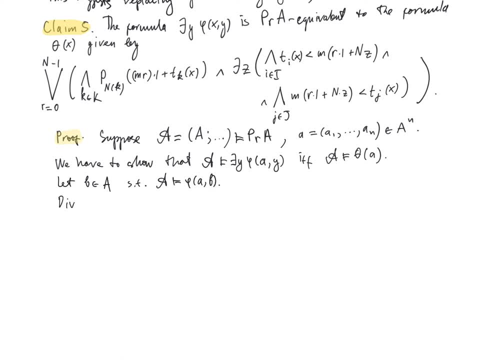 Then division with remainder, using the corresponding axiom of Pressburger arithmetic, yields some element C in the base set and some natural number R, such that we have: B is equal To R times 1 plus N times C, and the remainder R is greater or equal than 0, but less or equal than N minus 1.. 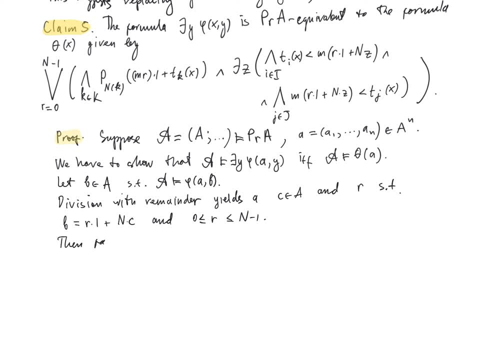 Note that then for K in K we have that M B plus T K of A is equal to M R times 1 plus N C plus T K of A is equal to M R 1 plus M N C plus T K of A. 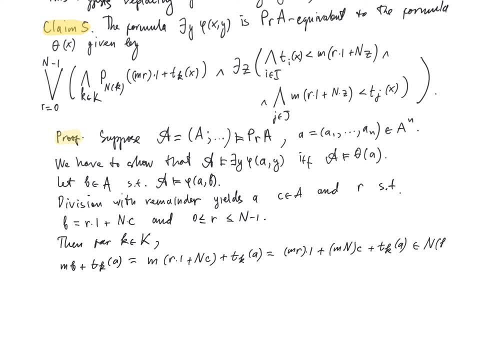 which belongs to the set N. In other words, this element in A is divisible by N of K, And so we have that A satisfies P, N of K, M R times 1 plus T K of A. and I recall, as usual, that whenever we multiply we don't actually have multiplication in the language. 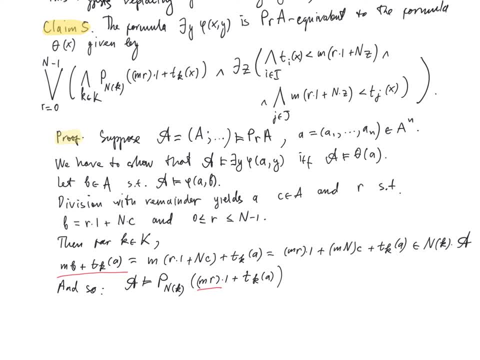 It just means an abbreviation for the sum corresponding number of times, And the data M, R is provided by the formula. It's not an element of the structure, And so we have A satisfies this divisibility condition, And also we have that T I of A is less. 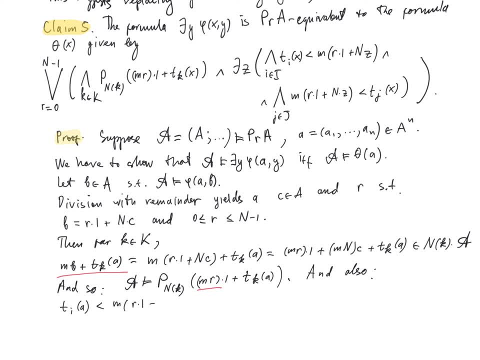 than M R times 1 plus N C for every I and I, And we have M R 1 plus N C is less than T J of A for every J and J. That's of course because R 1, plus N C is the expression for B in the structure. 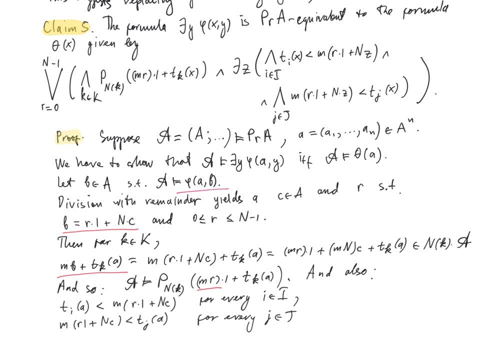 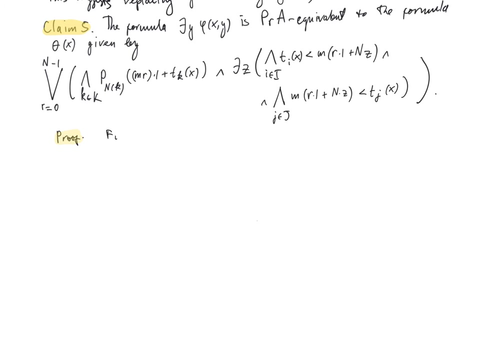 And we assume that B satisfies the corresponding formula. Hence this holds as well. So we conclude that A satisfies data of A with the existential quantifier exists Z, witnessed by C. For the converse, suppose that A satisfies data of little a, And since data is of course a disjunction of several formulas, 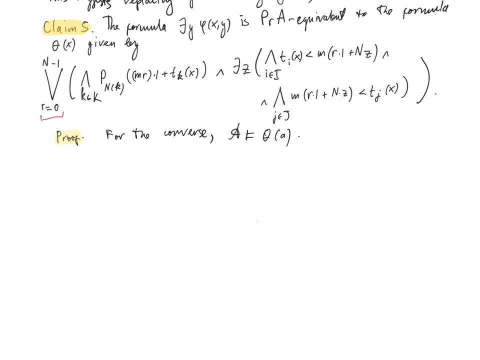 one of the, at least one of the disjuncts must hold. So let's say, suppose the disjunct of data of A indexed by R in 0 through N minus 1 is true in A with the existential quantifier. 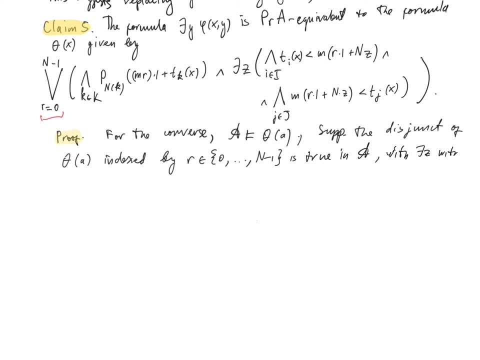 quantifier exists, Z, witnessed by some element C in A, then we can take B to be the element R times 1 plus N times C and by looking again at the formula we get that A satisfies phi of AB. just unwinding the formula in terms of the 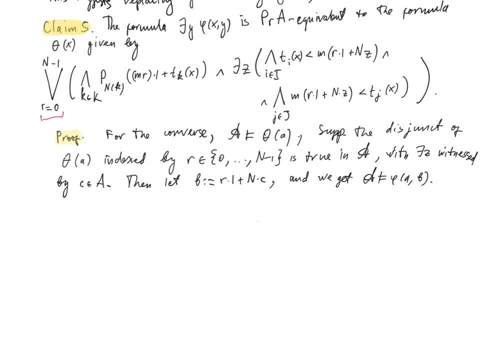 original formula phi. so this shows that theta is equivalent to exist Y phi of XY in Pressburger arithmetic, since the model A in which we were working was arbitrary. Looking at theta now, we see that this part is quantifier-free, so what remains is to: 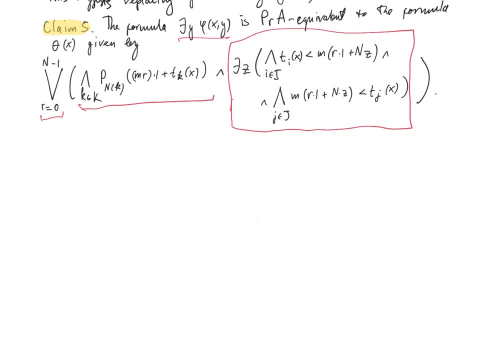 show that this formula exists. Z, etc is equivalent to quantifier-free one. So this means that we have reduced to the situation where H is equal to K, is equal to the empty set, of course possibly after choosing the notation. so this means that in our formula there are no equations and there are no congruences. 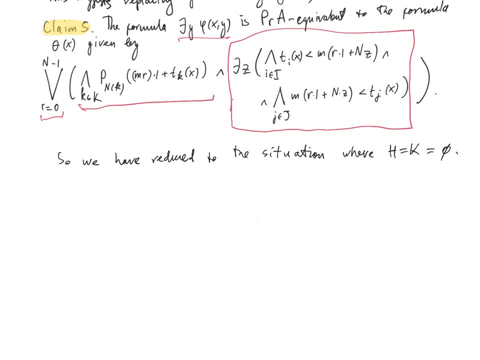 so we only have the inequalities. part ie phi of XY is of the form of the 0, i in i. t i of x is less than my and j in j. my is less than t j of x. in the case when j is empty set or i is equal to the empty set, then our function is the. 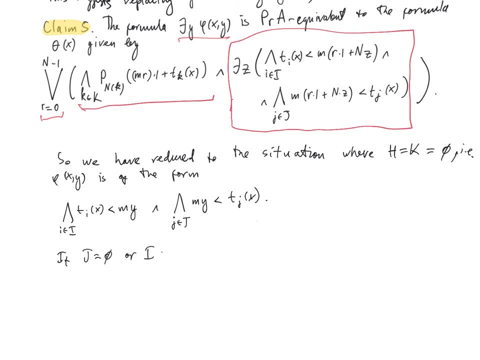 function i in x is equal to the empty set, then we have that presbyter arithmetic implies exists y, phi of x, y. Indeed, assume, for example, that j is equal to the empty set. then we are only concerned with the finite family of inequalities given by all i and i. 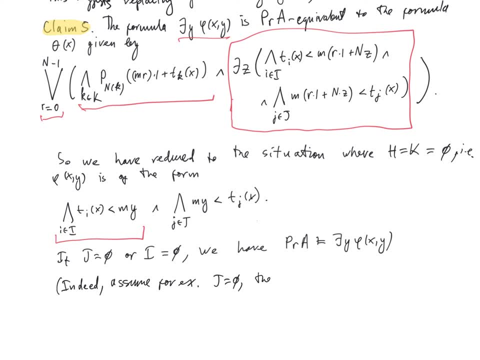 but then we would have that for any. a models, presbyter, arithmetic and a tuple in the base set of length n. we can consider the set t1 etc. So the set ti of a for i in i is finite. so just a finite set of elements in the structure. 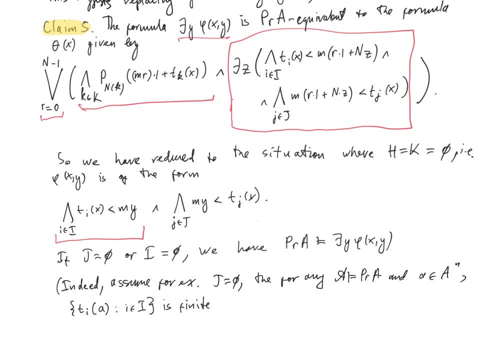 but of course the underlying linear ordering of the structure has no largest element. so we can always find some b which is greater than all of the elements of the set. so if we call this, for example, t, some b in a which is greater than all of the elements in the set. 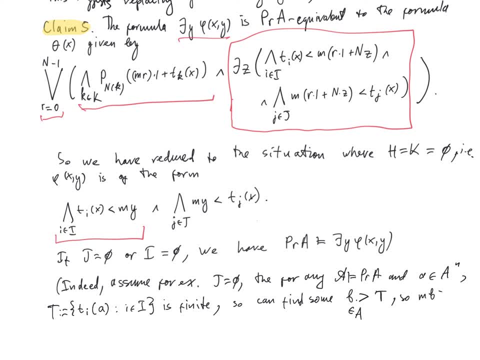 so of course also mb is greater than all of the elements in the set, and so a satisfies phi of ab for any choice of the tuple. So indeed, presbyter, arithmetic implies exists y phi of x. y in this case, The case when i is empty, is symmetric. just have to pick an element smaller than all elements in a. 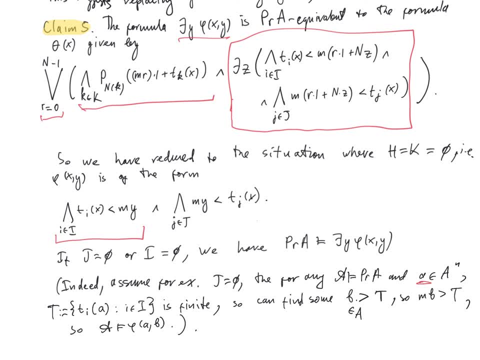 given finite set, and so by our convention on quantifier elimination- in this case we see that presbyter arithmetic implies- exists y phi of x, y if, and only if, x is equal to x. so we obtain a quantifier-free formula equivalent to this: 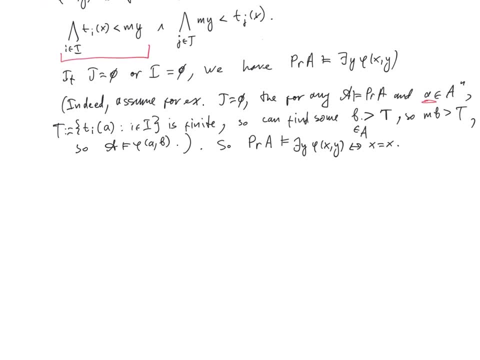 Hence we have claim 6, we may assume that both i and j are non-empty. if a is a mode of presbyter arithmetic, Now let a be a module of presbyter arithmetic. with the underlined set a, then for each choice of tuple a in a to the n. 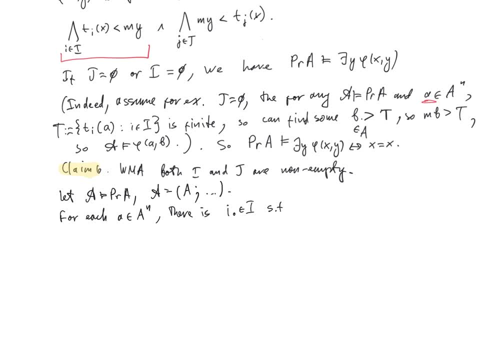 there is some i is zero in i, such that the element ti0 of A is maximal among the elements of the form ti of A with i in I. and also there exists j0 in j, such that tj0 of A is minimal among the elements tj of A with j in j, simply because both are finite sets. 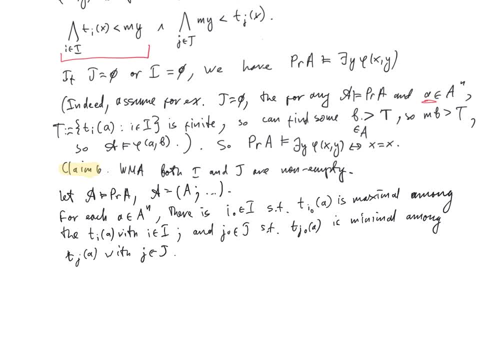 so we can choose one, One which is maximal and one which is minimal. And, moreover, each interval of m successive elements of A contains an element tj, tj, tj, tj Of ma, so contains an element divisible by m. So it just follows from the axiom of Pressburger arithmetic. 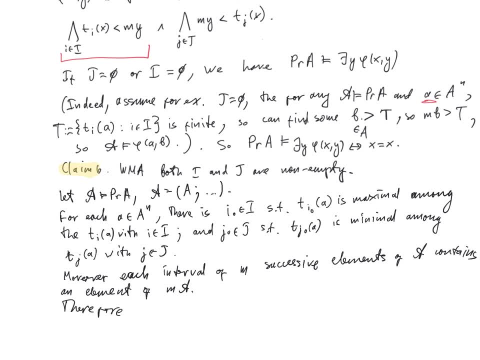 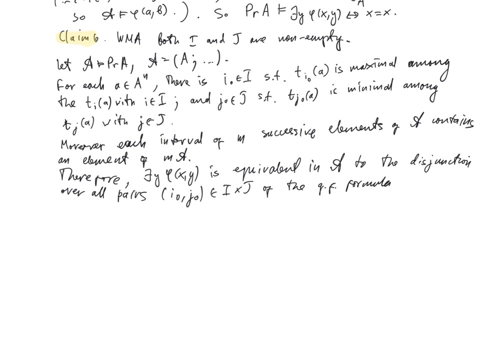 Therefore we have that the formula exists. y phi of xy is equivalent in A to the disjunction over all pairs i0, j0 in i times j of the quantifier-free formula given by the following expression: So we have the conjunction over all i in i. 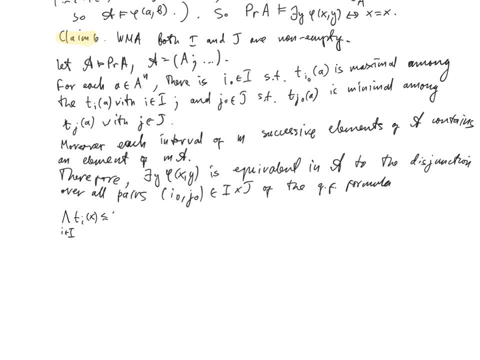 ti of x is less or equal than ti0 of x and the conjunction over all j in j is less or equal, then tj of x and the conjunction over all r from 1 to m of t i 0 of x plus r 1 and t i 0 of x plus r 1 is less than t j 0 of x. 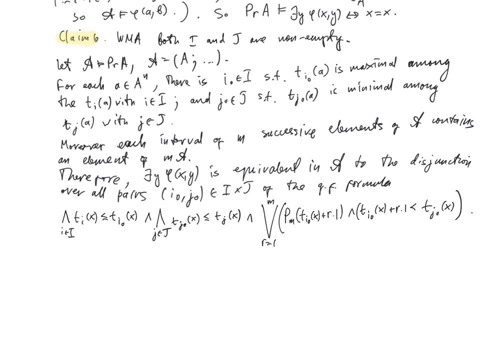 So, namely, since we always know that in any interval long enough, namely an interval of m successive elements, there exists an element divisible by m, then exists y, phi of x, y, which expresses a number of linear inequalities with coefficient m. indeed, can be written as this: 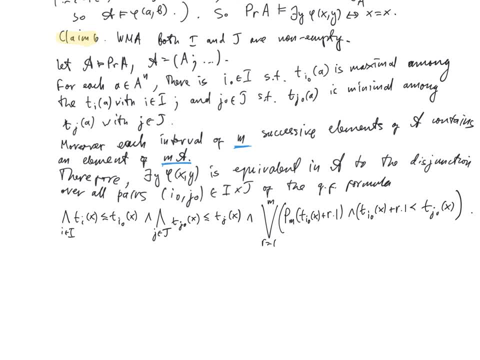 the disjunction of the role pairs i 0, j 0, because we don't know in advance for a given a, which t i and which t j 0 are going to witness the maximal and the minimal elements respectively. but there will be some choice for which they will be the maximal and the minimal one, and hence for that 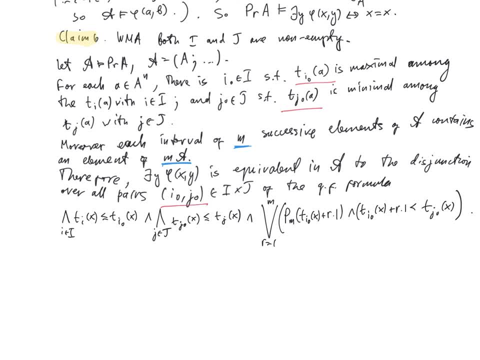 choice, the correspondence disjunct is going to be satisfied And of course if one of them holds, then the formula exists: y, phi of x, y also holds, So this completes the proof. Note that whenever we write less or equal in this expression, of course it's not part of the language, so we use it as an abbreviation. 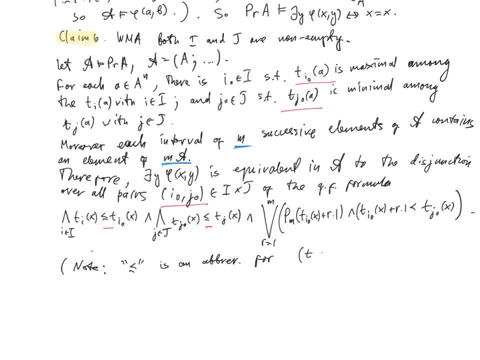 for the formula t is so if we write, for example, t is less or equal than t prime, this abbreviation for t is less than t prime or t is equal to t prime. Okay, so this completes the proof of consciousness. Let's do the next one. 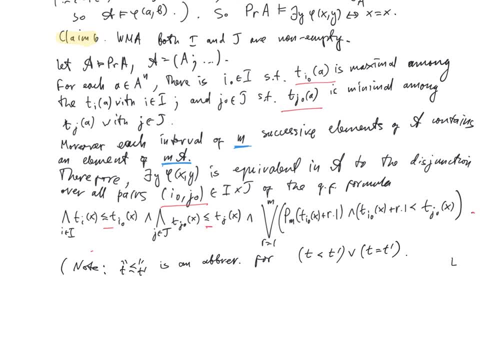 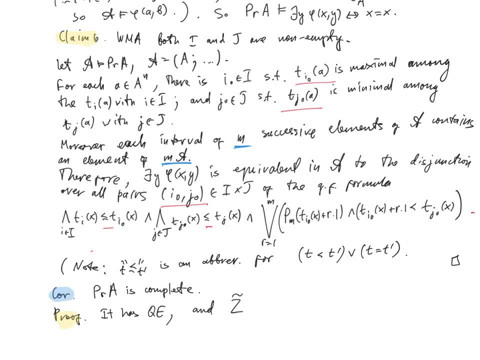 And, moreover, the standard model Z tilde, which is the integers with addition and divisibility by n for the predicates P, n, embeds into every model of Pressburger arithmetic. So namely, we can just look at the interpretations of the symbols 1, one plus one, etc. and also the inverses. so this gives us a copy of z tilde inside of any model of. 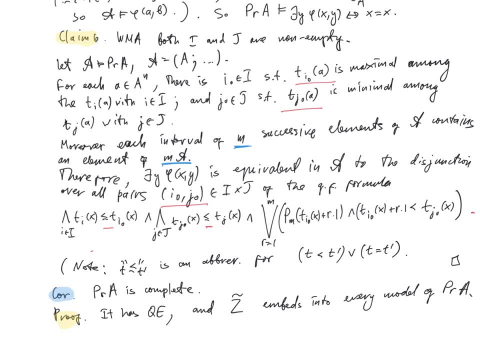 presberger arithmetic. and then we know by the general criterion for completeness of a theory that presberger arithmetic is a complete theory. note that, unlike in the case of algebraically closed fields, we have not used the semantic criterion for quantifier elimination here, but rather were really explicit about how to obtain.